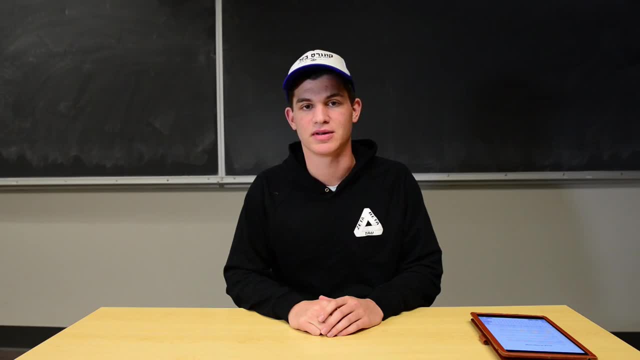 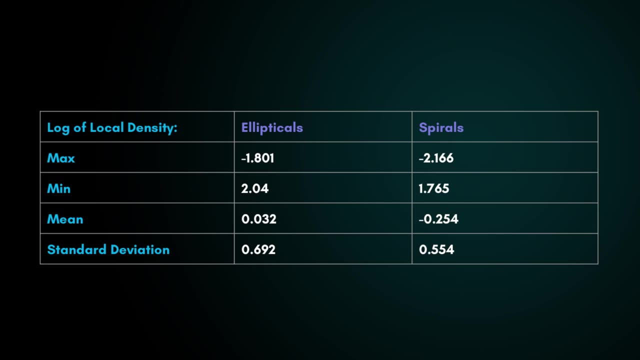 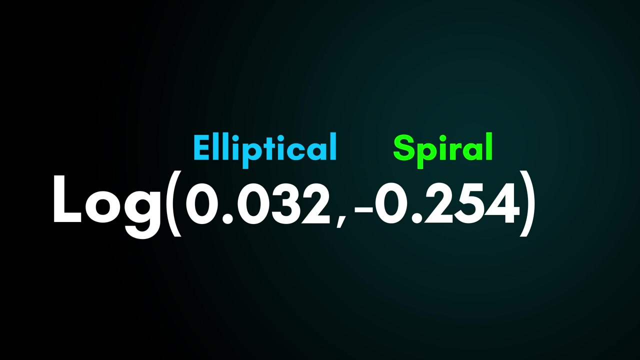 To test this theory, we pulled the local density data from Galaxy Zoo for galaxies that over 80% of people identified as being elliptical. Using the summary stats helper, we assembled this chart of the density data and found the averages. Now, remember, Galaxy Zoo density data is in log form. 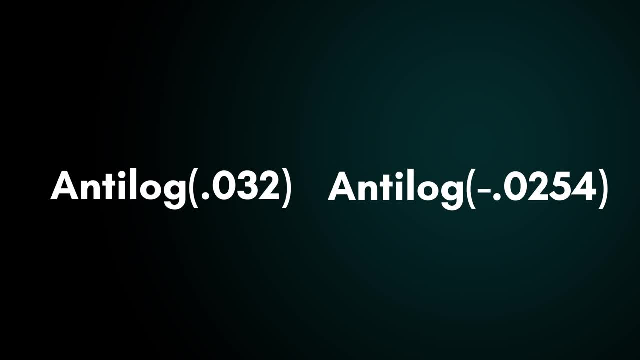 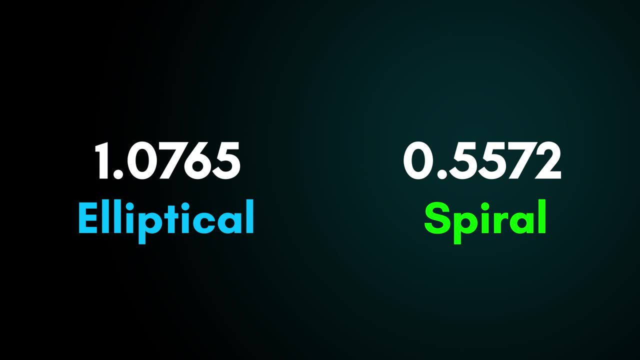 so we took it out of log form using the antilog function to compare them more easily. From that we get an average of 1.0765 for ellipticals and .5572 for spirals. That means that ellipticals are, on average, located in areas of the universe. 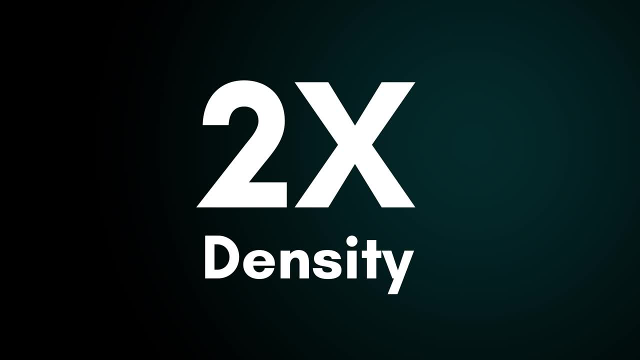 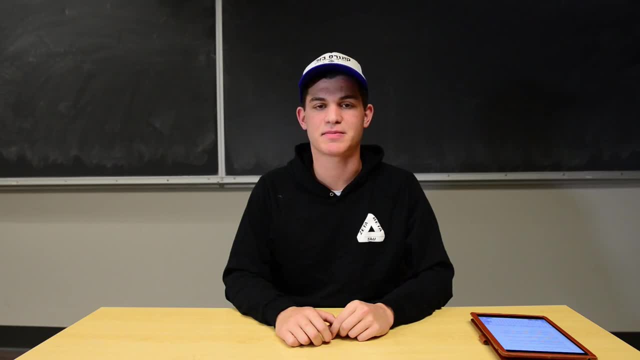 that are about two times more dense than the areas in which spirals are found. That was a good start, but we wanted to go deeper, So we made a histogram of elliptical galaxies and spiral galaxies, as they relate to the density of the environment that they are in. 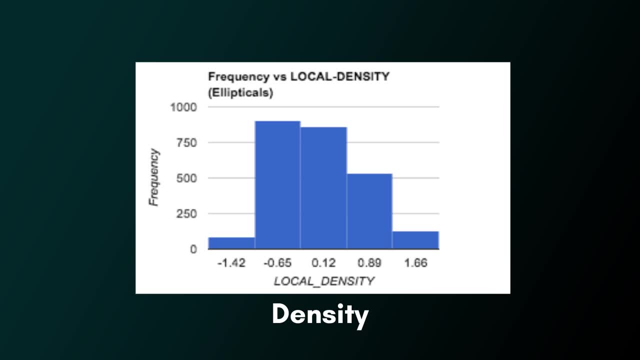 On the x-axis we have the distribution of log densities, Just like a histogram with a linear x-axis. the more right a point is on the histogram, the denser it is. The y-axis shows the density of the environment and does not show the density of the environment in the frequency. 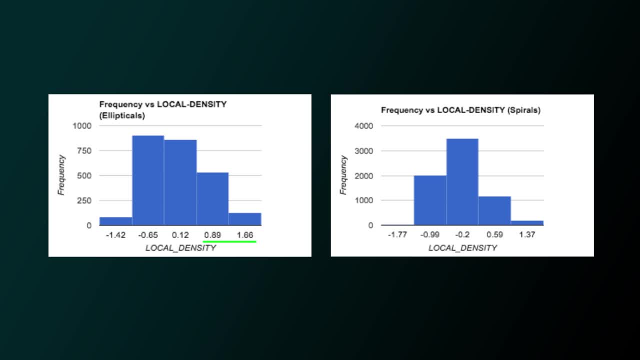 Though there are less elliptical galaxies than spiral galaxies in the dataset, we can still see that ellipticals occur in high-density areas. We can also see that galaxies occurring in maximum density areas are ellipticals. When we compare both the graphs, it becomes evident that for ellipticals, 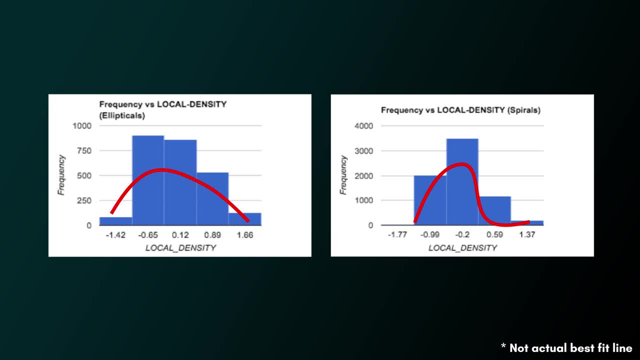 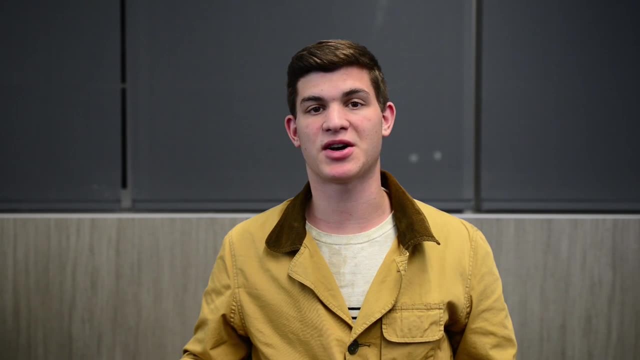 the density distribution of galaxies lies in the denser region in comparison to spirals. We can see this from the histogram bars from both of the graphs. only is the maximum density higher for elliptical galaxies, but so is the mean. After looking at images online and in the Galaxy Zoo dataset, we began to 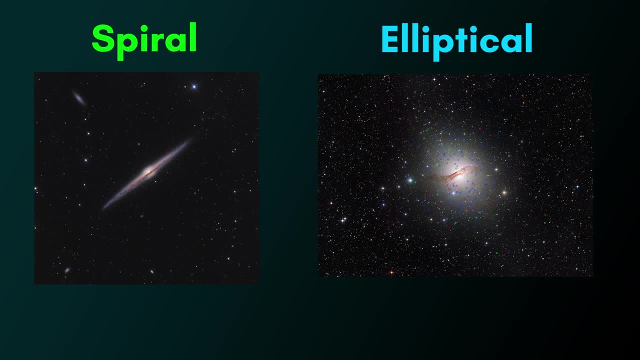 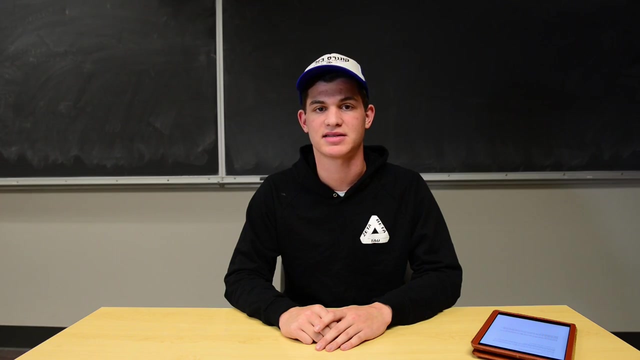 notice a pattern: In most images of elliptical galaxies, they appear to be surrounded by other galaxies, while in most images of spiral galaxies they appear to be distinctly separate. While we can't predict what would happen if we used a dataset larger than the one given by the Galaxy Zoo, all the evidence on 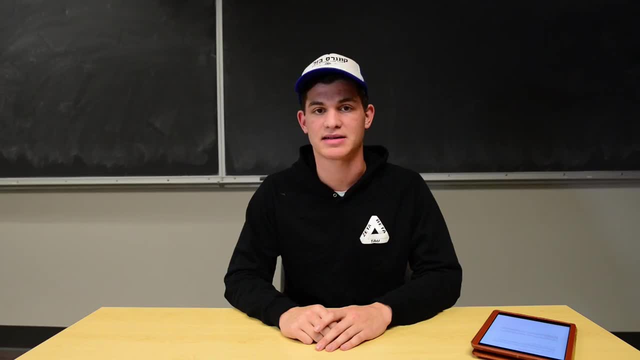 hand would suggest that our hypothesis is correct that elliptical galaxies are most likely to occur in the highest density areas of the universe.